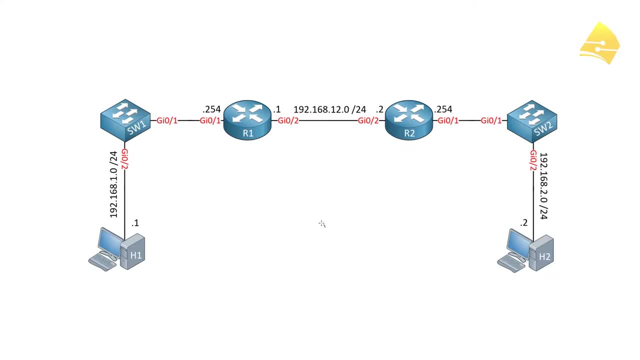 is connected to R2, switch2 and then host2.. Now let's say that we are trying to troubleshoot an issue where host1 is unable to reach host2.. So there is no connectivity between these two devices. Now let's say that we are the administrator of R1. So I will try to figure. 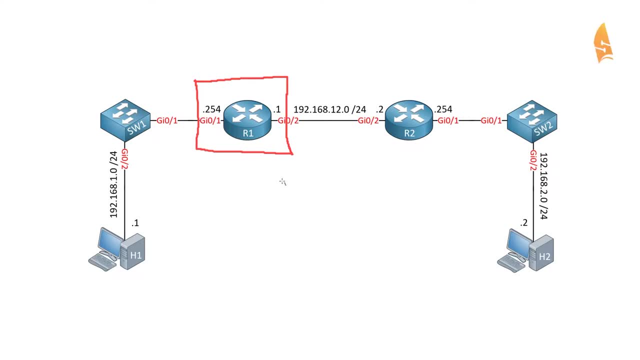 out what the issue is mostly by looking at R1.. Only when I'm unable to fix it from R1 I will look at some of the other devices. So let's take a look at R1. And the first thing I'm going to try is see if I can ping host2. 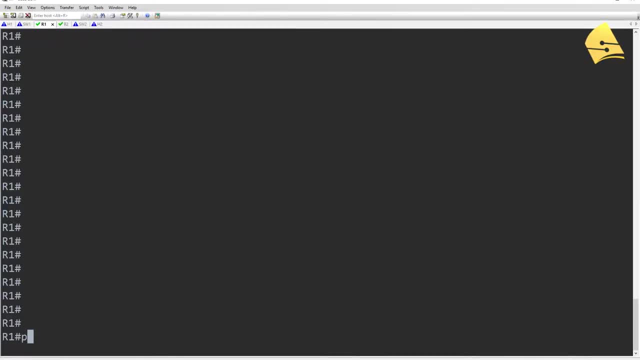 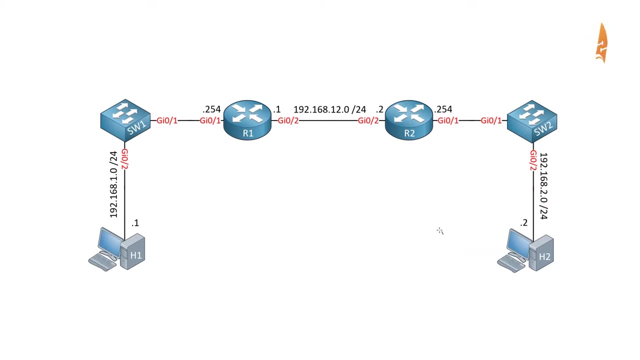 from R1.. So let's go to R1 and let's just try a quick ping Now. this ping is failing. So what I should do now is try to ping the device or the IP address that is one step closer to R1.. So that would be R2 over here. So that is 254, that's the address from the. 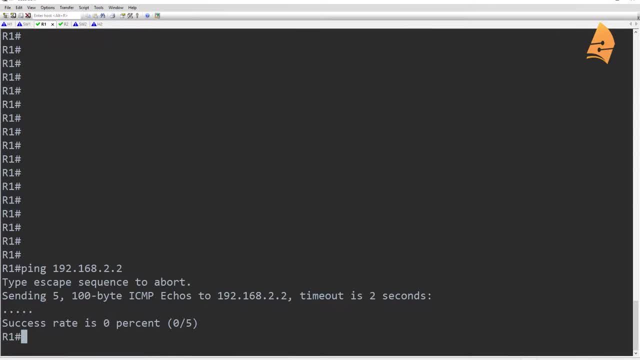 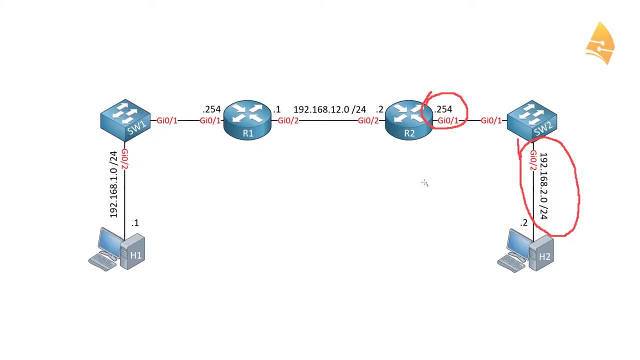 same subnet as host2 is in, So let's give it a try Now. this ping is also failing, So right now there are two options, or there are three options. basically, There could be something with this link over here. So maybe this link is not working, Maybe R1 doesn't. 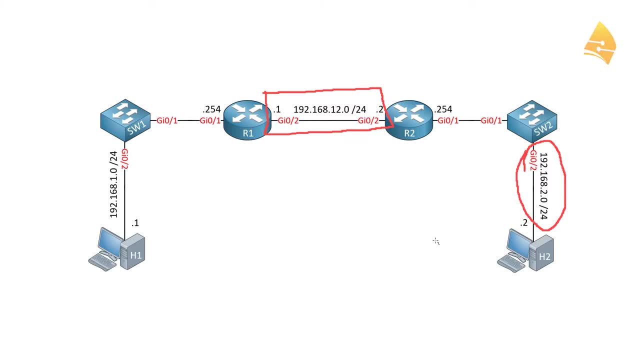 know how to reach this network, So that would be a routing issue. The third issue would be that it's possible that R2 is not able to reach this network, So that would be a routing issue. The third issue would be that it's possible that R2 is not able to reach. 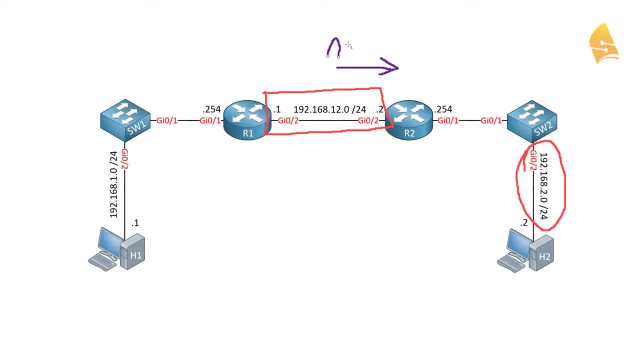 this network. So that would be a routing issue. The third issue would be that it's possible that R2 has an access list. So an access list over here, Maybe inbound, which is filtering these packets. Trying to figure out if it's an access list can be difficult. 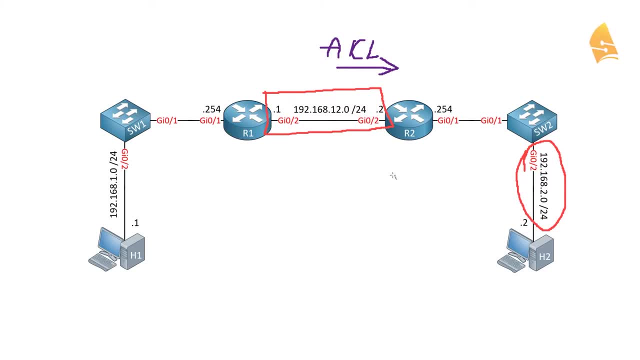 Cisco IOS, when you have an access list and it's dropping a packet, then the router will respond with an ICMP unreachable message. But most firewalls they will just silently drop your traffic. So what I will do first is I'll do a quick ping to see if this link. 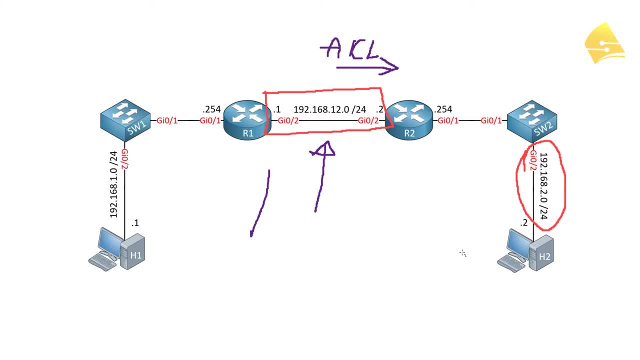 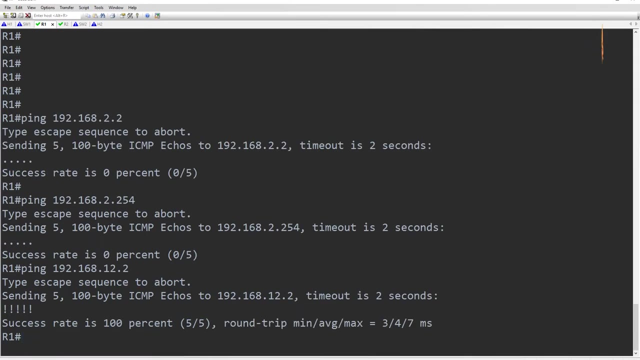 is working, So the link in between R1 and R2. And if not, I will see if it's a routing issue, because that's something I can check from R1.. So let's go to R1. And you can see that I can ping the IP address of R2.. 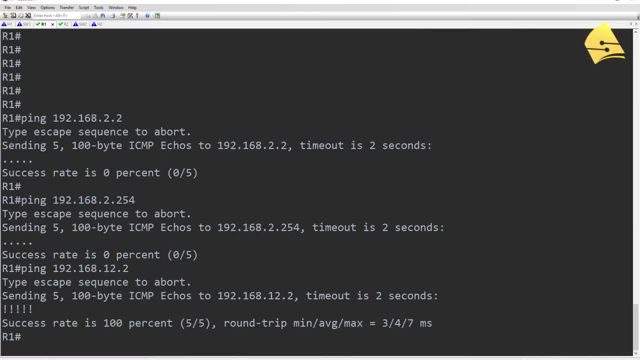 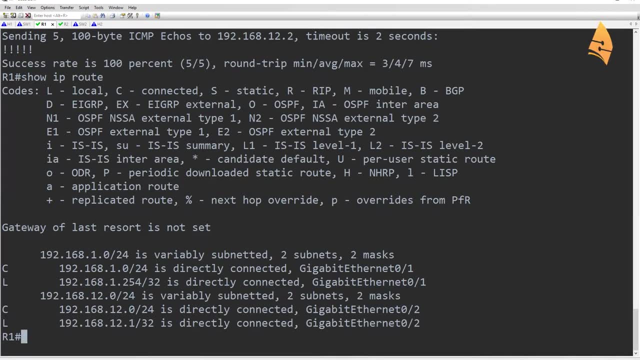 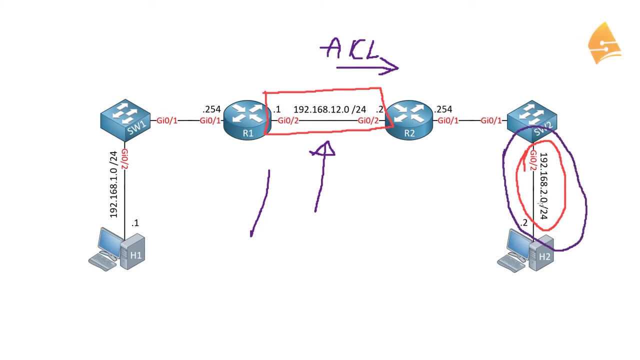 R1. The IP address of R2 on the directly connected link. So let's see if this is a routing issue. When we look at R1, you can see that there are no routes at all, Just the directly connected routes. So R1 doesn't know how to reach this network over here. So the 192.168.2.0. So. 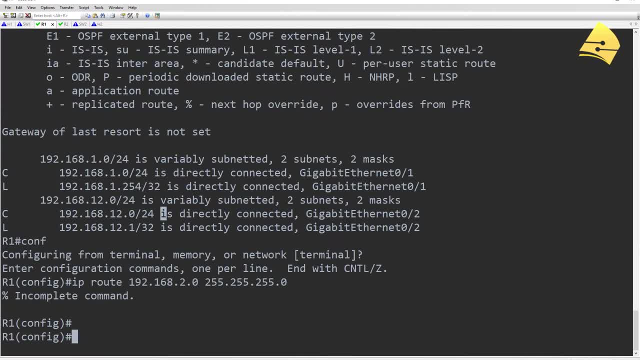 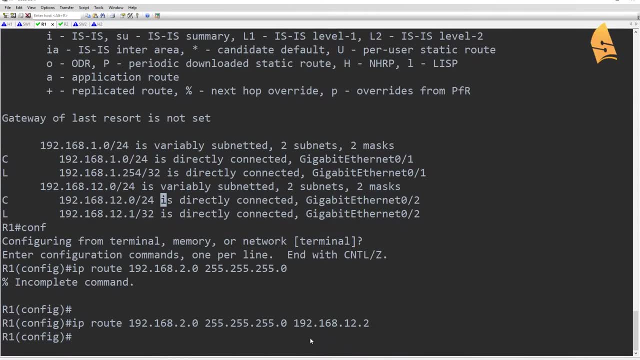 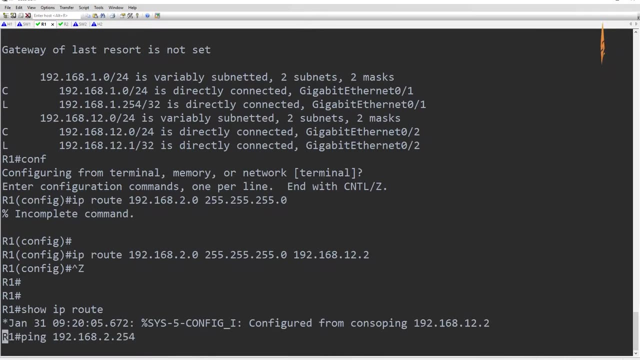 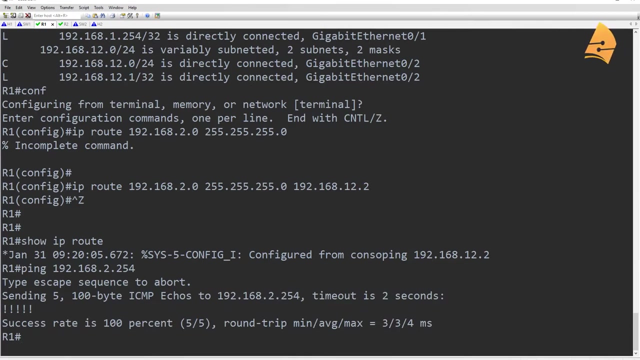 let's add a route here: R1.. R2. And the next hop will be 12.2.. That's the IP address of R2.. So with this route, let's see if we can ping this address now. So this is now working, So we can ping the R2 address. 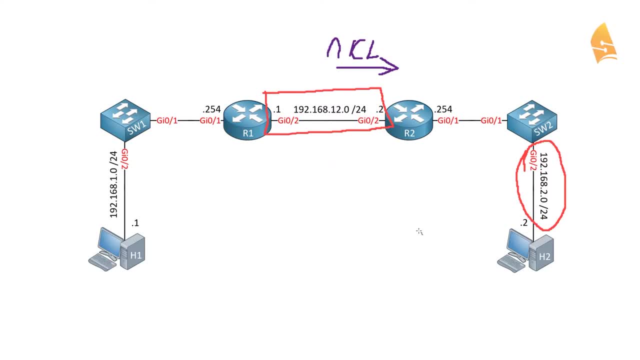 Let's see if- Let me clean this up a bit- R1. R2.. R2.. R2. R2.. So right now I'm able to ping this IP address. So now let's see if we can ping this address. 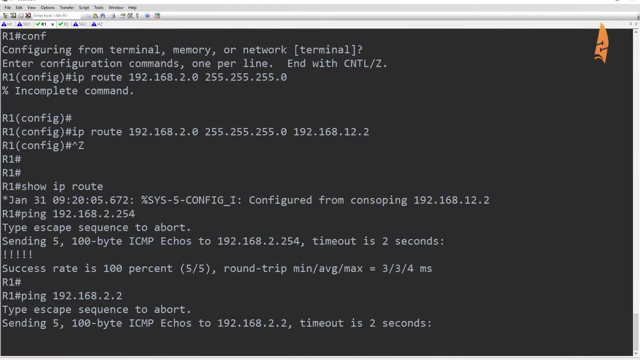 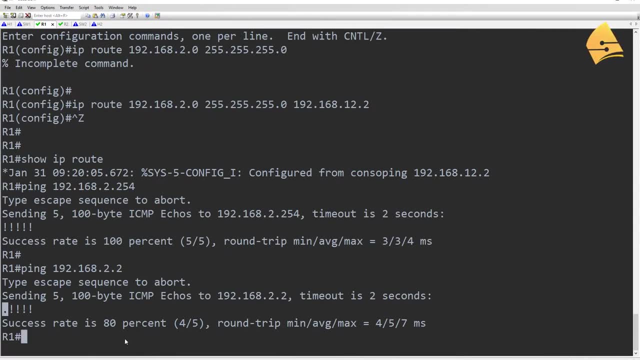 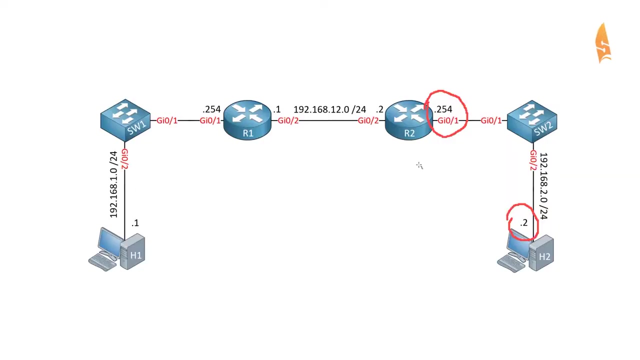 over here And we can see it's working. The first ping is failing. That's probably because of an ARP request in reply. That takes some time, So that's where you get a timeout, But this is now working. Since this ping is working, that also tells me that host2 has a default. 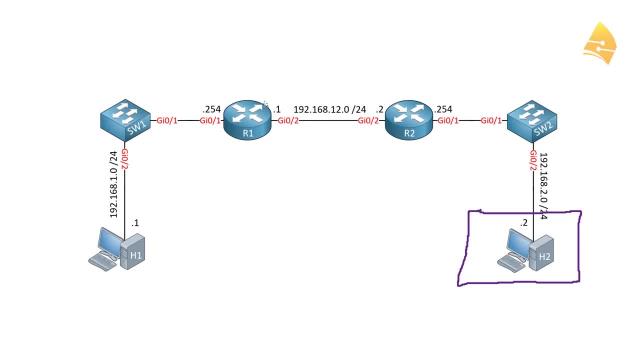 gateway, Because when R1 is sending this ping, it's doing so from this IP address over here .1. from this subnet over here- the 12.0.. And because this IP address is not in the same subnet as host2, host2 will have to use its default gateway in order to reply to this. 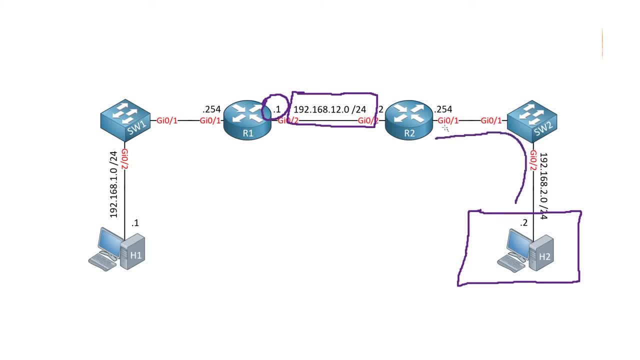 address. So host2 will have to send it to R2 over here. So since host2 is replying to this ping, I know that it has a default gateway. So so far, so good. So right now we know that this part over here is working as it should. 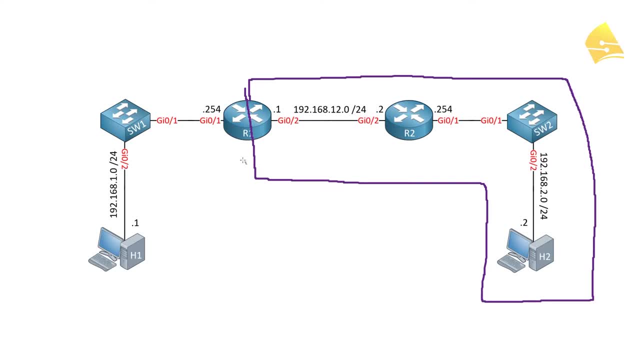 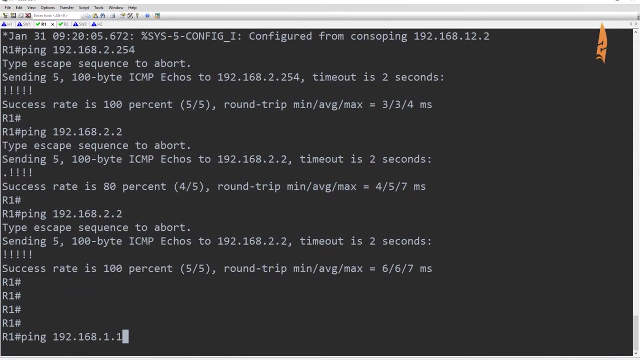 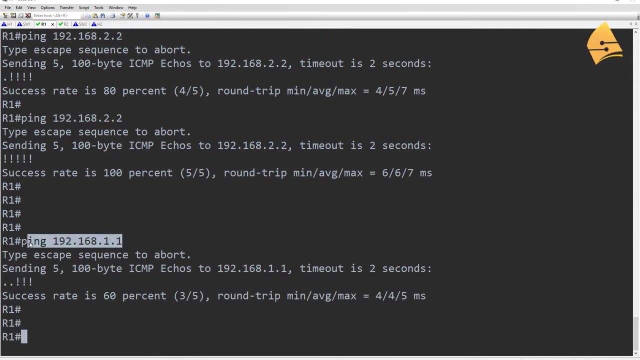 .1.. Okay, So what I'll do now is let's see if I can reach host1 from R1.. So we'll just do a quick ping to this direction And we can see this ping is working. So two timeouts because of ARP and now it's working. 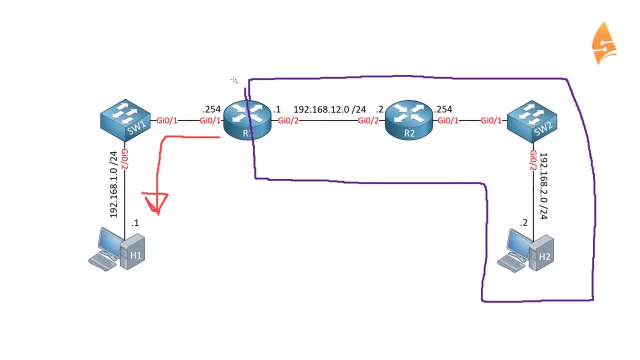 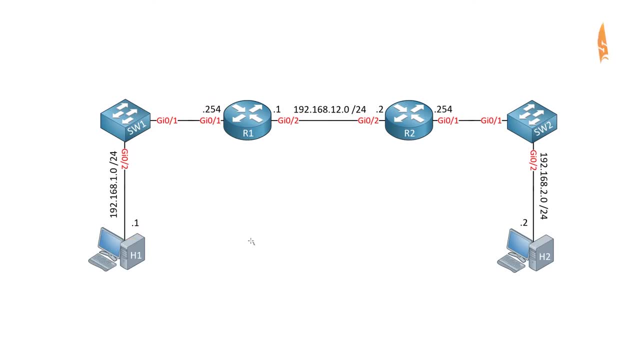 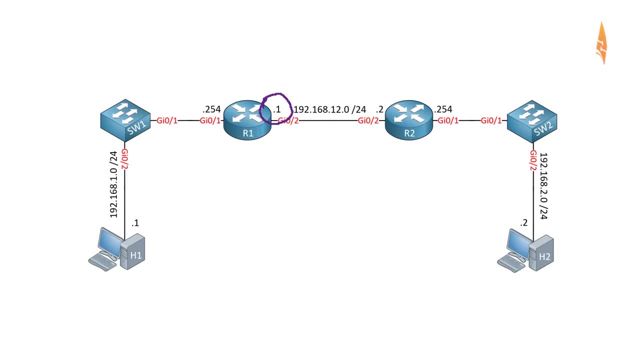 over here from 12.1.. And if I send a ping from that source to host1, then host1 will receive a ping from a source outside of its own subnet And it will have to use its default gateway to reply. So let's see if this ping is working or not. 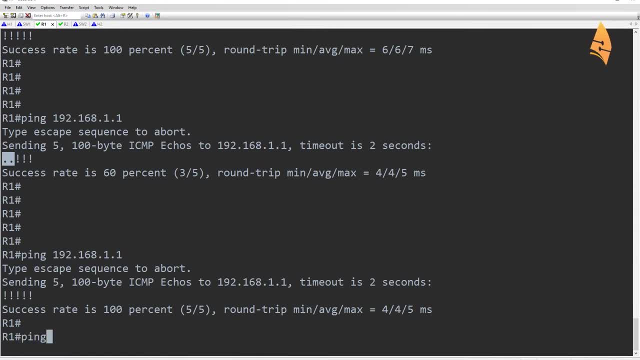 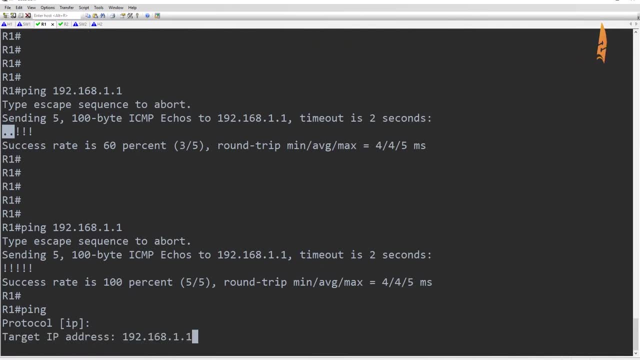 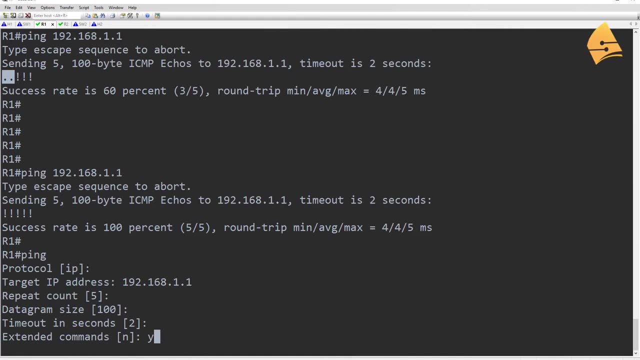 So what I'll do if you use the ping command. we need to use the extended ping command. Just hit ping. enter target 1.1, repeat count 5, size is fine, timeout, this is all good, but we need the extended commands. 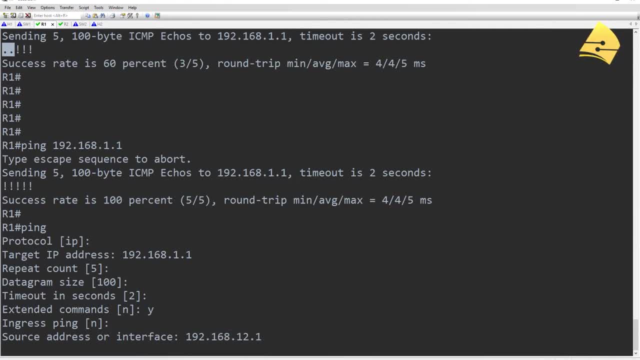 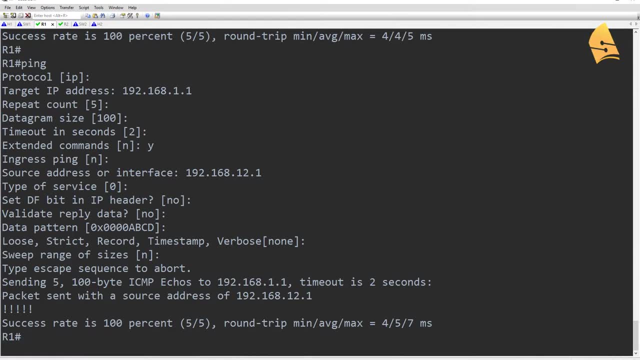 And here you can specify the source IP address, So 12.1.. We don't need any of the other settings. There we go. So we got a ping from 2.1.1,, from 12.1, and this ping is working. 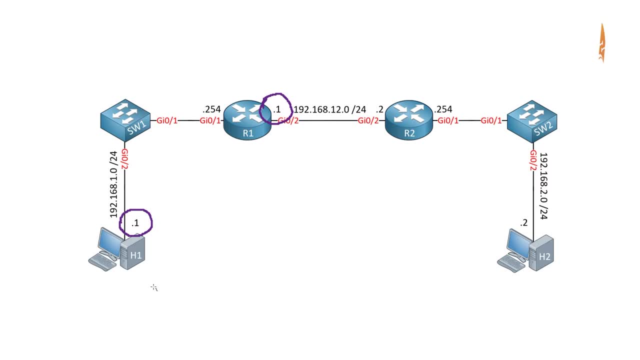 So that tells me that host 1 has a default gateway. Okay, so so far, so good. I can use the same logic to figure out if host- sorry, R2 has a route or not. So I know that I can ping from this IP address to this IP address. 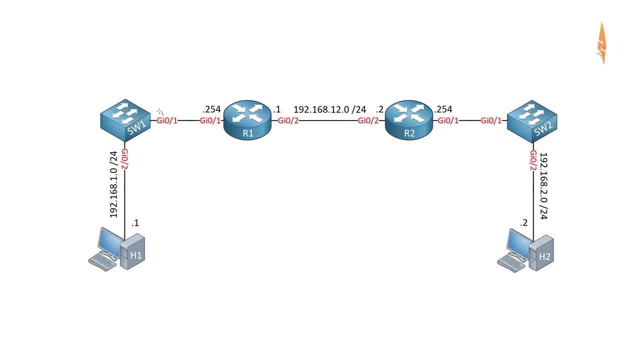 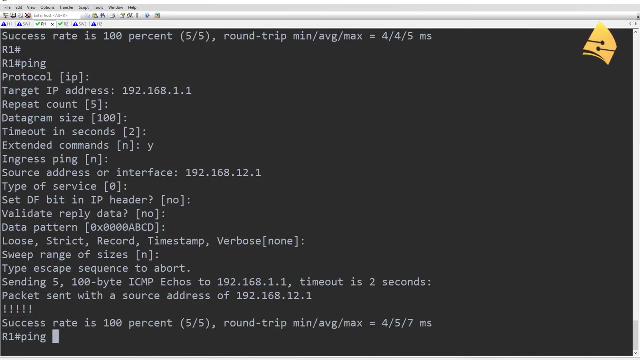 But I don't know if I can ping from this IP address, which belongs to this subnet, To 2 or maybe one of the IP addresses of R2.. So let's give this a try. So I'll go to R1 and we'll start with host 2 and instead of using the ping command without. 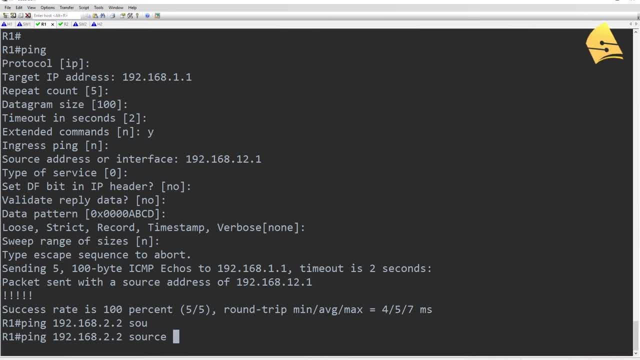 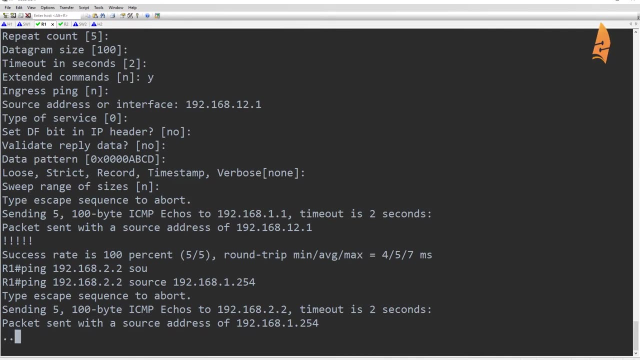 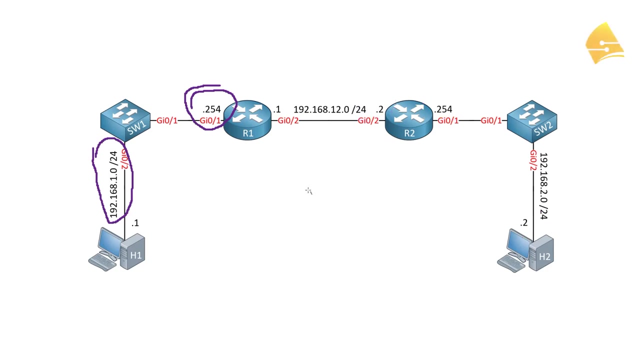 any parameters and hitting enter, you can also do it like this, which is a bit quicker. So to 2.2 from 1.254.. So let's send this ping. This ping is failing, So I'm unable to ping host 2.. 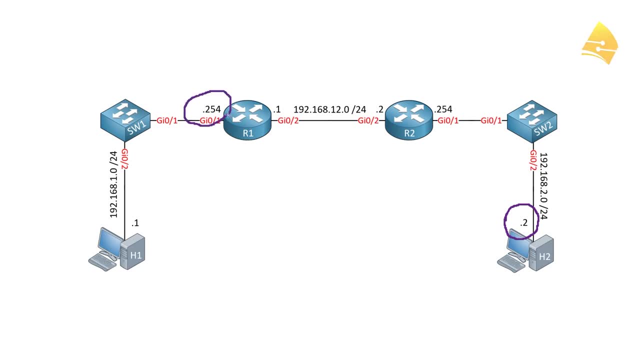 So this is the destination and this is the source This ping is failing. But when we try this Instead of ping it with this address as the source, it was working. So this tells me a lot. Well, there are two options here. 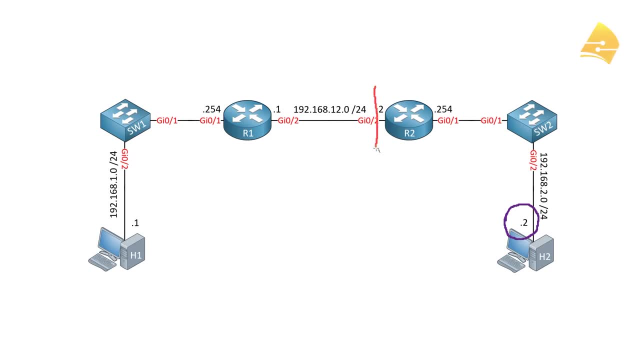 Option 1, R2 over here. So R2 maybe doesn't know how to reach this network over here, So that's an option. The other option could be that there is an access list somewhere filtering and dropping this traffic. So which of the two options it is that will be difficult to figure out from R1.. 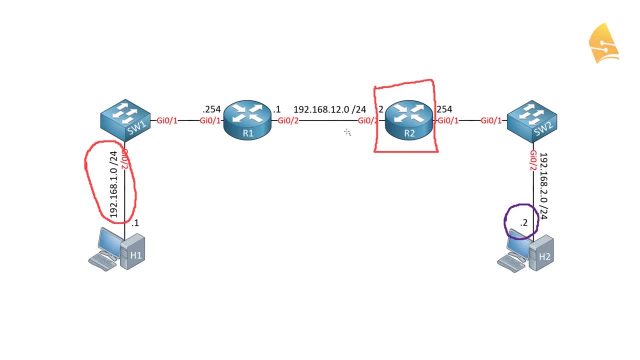 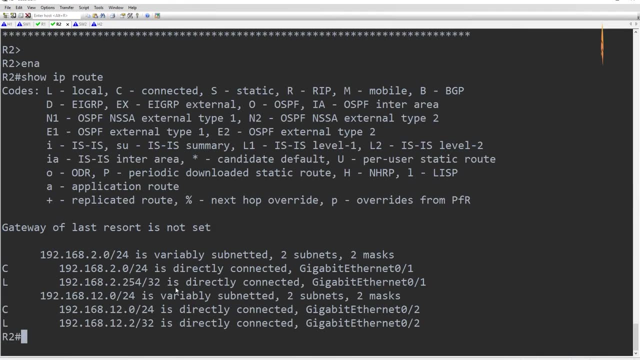 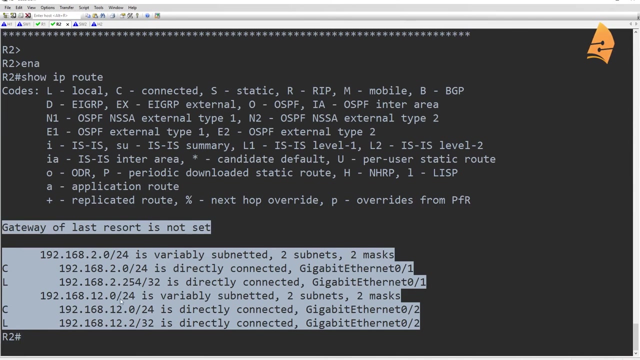 So this is something that I do have to check on R2.. So let's go to R2 for this And I'll just check its routing table, And what we see here is that it only knows about directly connected links, So it has no idea how to reach the network that is behind R1. 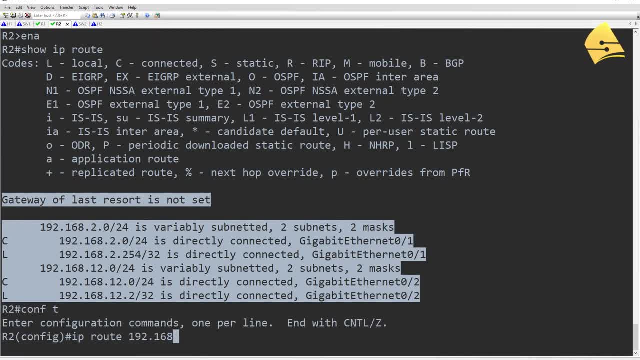 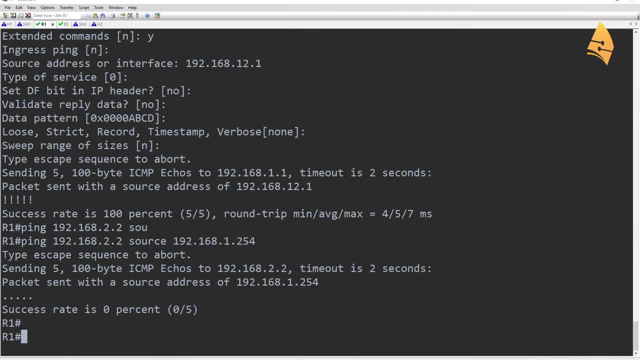 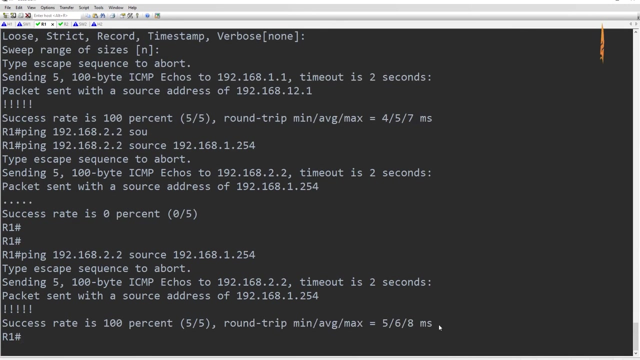 So that's something that we have to solve. So to reach 192.168.1.0, we go to 12.1.. Like this. So let's try that. ping again now To host 2 from 1.254.. 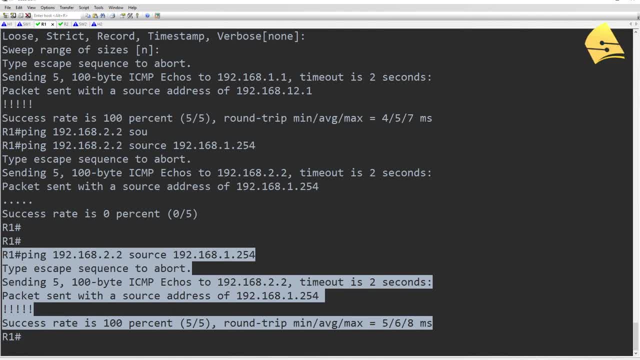 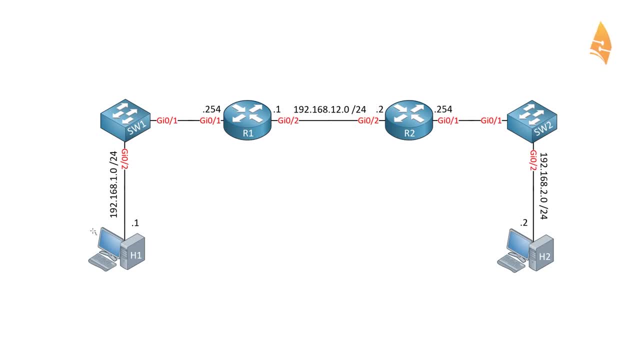 And now we can see that this ping is working. So that's something that we have to solve. So to reach 192.168.1.0 we go to 12.1.. So the only thing left to try is see if I can ping from host 1 to host 2.. 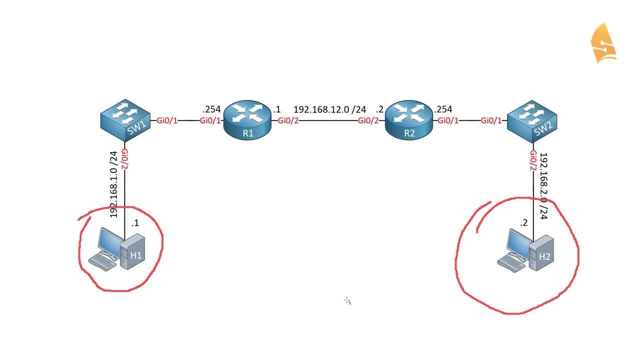 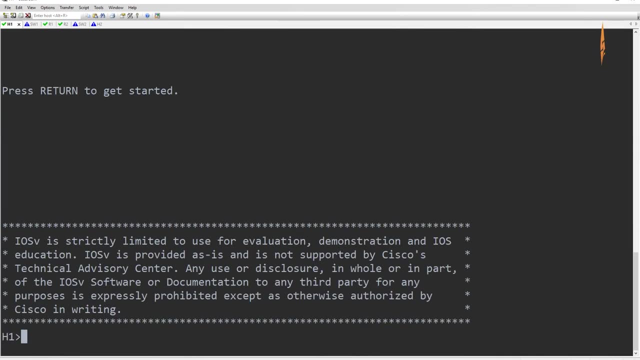 Because basically everything that I can try from R1 we have done, So there's nothing left to try here. So I'll go to host 1 over here And we'll see if I can ping to 2.2.. Which is working. 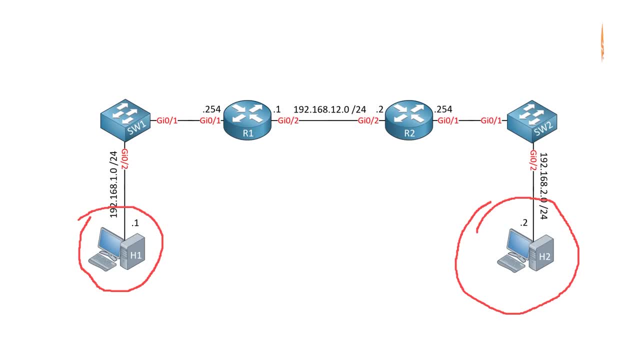 Okay, So that's how we solve this issue. Okay, so that's basically it. So this is how you can use the ping command to troubleshoot or isolate some of your network issues. I hope this has been useful. Thanks for watching this video and till next time.